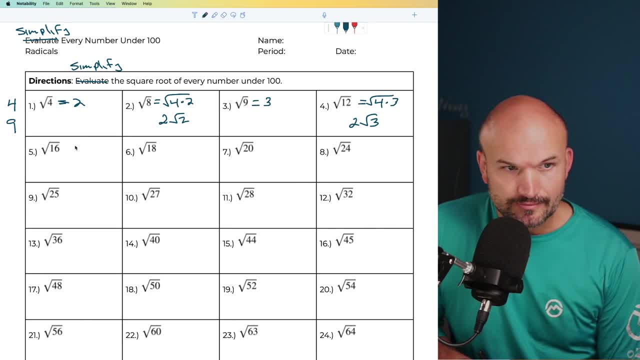 which is now going to lead me to a two square root of three. The next one here hopefully recognize that as a square number. that is going to be a four. So that is going to be the next square number that I'm going to write out, Then the next one, eight. we would say: all right. 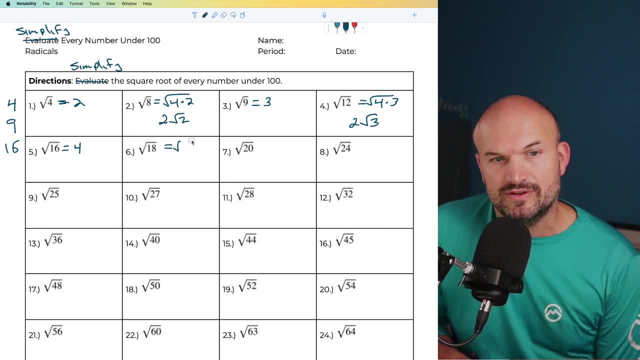 which of these square numbers can I rewrite that as a product And you could see that, hopefully, that is going to be a nine times three square to nine is going to be a three square root of three square to 20.. I can rewrite that as a square root of four times five. Now, the one thing I want you. 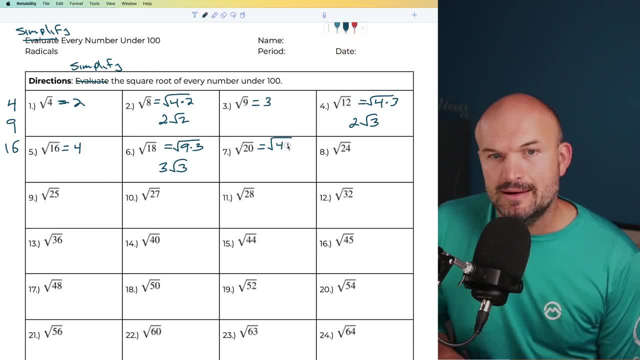 to notice is: I'm always trying to write this square number first. You don't have to do that, but in my opinion I like to kind of always try to try to do that first, just to try to remain consistent. So the square root of four is going to be a two square root of five for the square 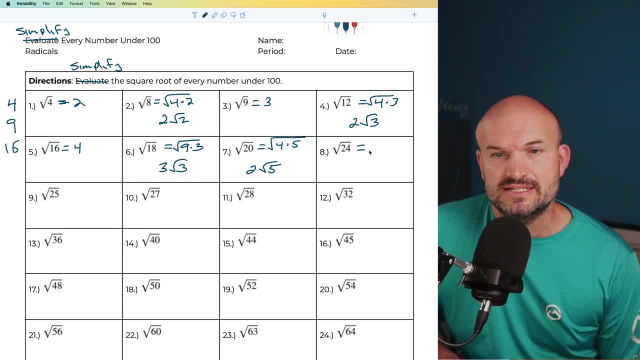 root of 24.. Uh, let's see that looks like that's going to be a four times six, So I can rewrite that as a four times six And therefore that's going to be a two square to six, the square to. 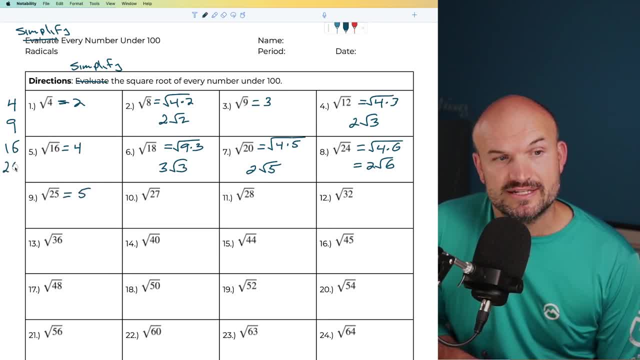 25.. That's going to be another square numbers. That's going to be five. So I'll say: all right, that's another square number here, 25 for 27.. Um, notice, a lot of times when they end in odd, you're going to be thinking of the nine. 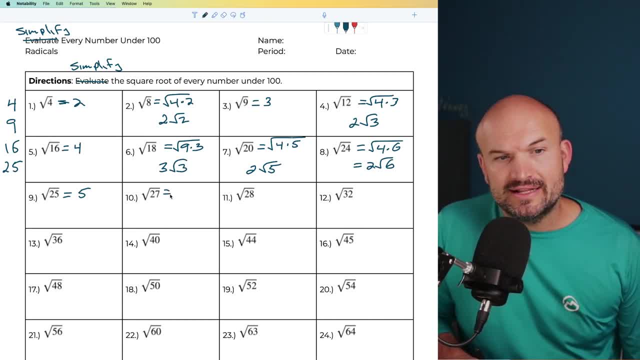 right, Because nine is my odd square number here, So therefore I can rewrite that as a square root of nine times three. I can take the square to nine, right, Because that's a square number, So therefore that's going to be three square root of three, uh, for 28.. It looks like that's going. 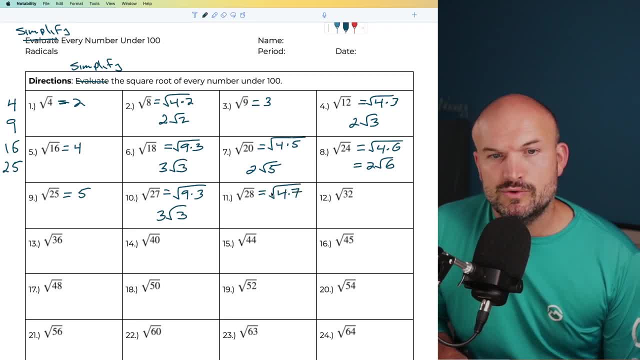 to be a four times a seven right. So four times seven square to four is going to be a two. And then I just have to leave the square to seven under the radical right, Cause you can't do anything with it. So you, therefore you have to leave it there. Uh, for the next one here. 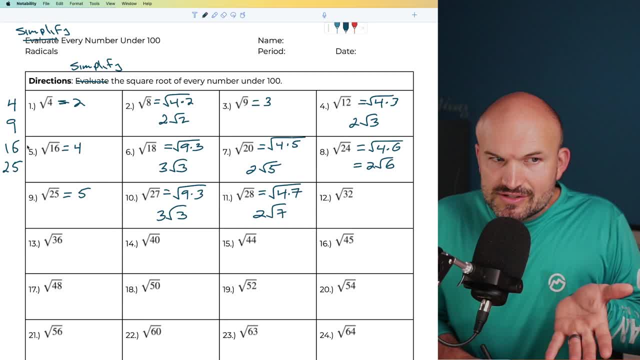 again one thing you could say: well, this is four times eight, right. But you can also say this is 16 times two. So which one do you choose? Well, technically, you can get to the right answer- choosing both- But I always like to do it. the way that I tell my students is always choose the. 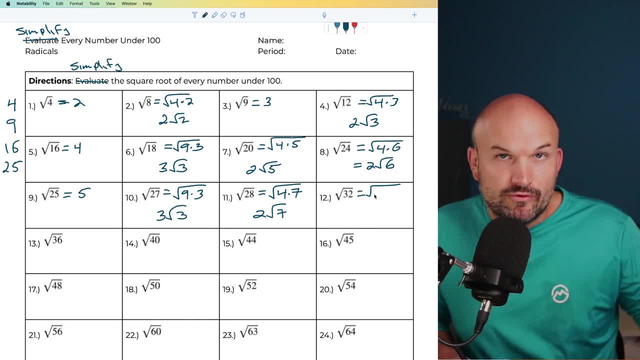 largest square number to rewrite as your product. So, rather than doing four times eight, I'm going to write this as a 16 times two. the square root of 16 is going to be a four. square to two. It just makes life a little bit easier, And so, therefore, you don't have to do as much work. Square to 36. 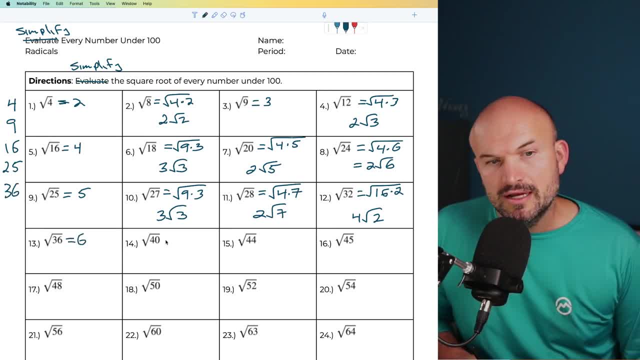 is a square number That's going to be six, So I'll go ahead and list this over here: Um square. looks like that can be a um square root of four times 10, right, You can just rewrite it in that. 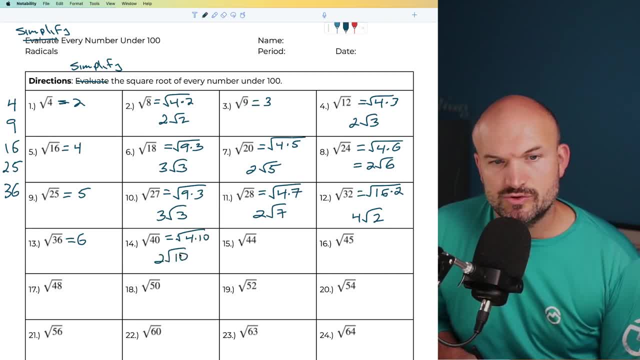 regard, Then I could take the square to four and square to 10.. So therefore, let's give me two square tens. My final answer: uh, for 44, it looks like I could do a four times 11.. The square to 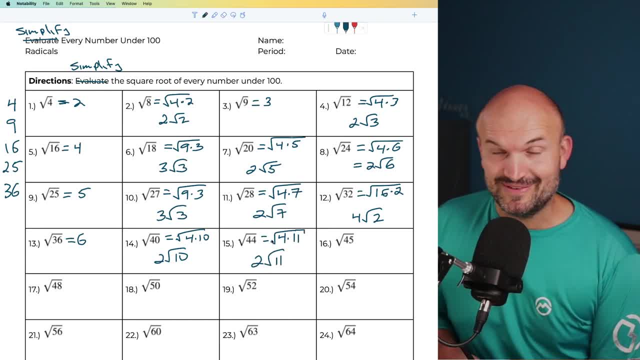 four is going to be two, And then we have 11.. You can see we're using four quite a bit right. So again, as you get through this, like the better and better you're going to get. uh, let's see 45.. 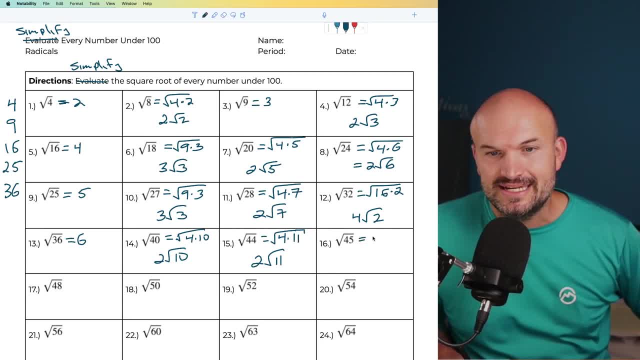 And again it's an odd number that makes me think of three or of nine, And indeed that is going to work. It's going to be a nine Or non. a nine times five square to nine is going to be three times the square root of five. uh, 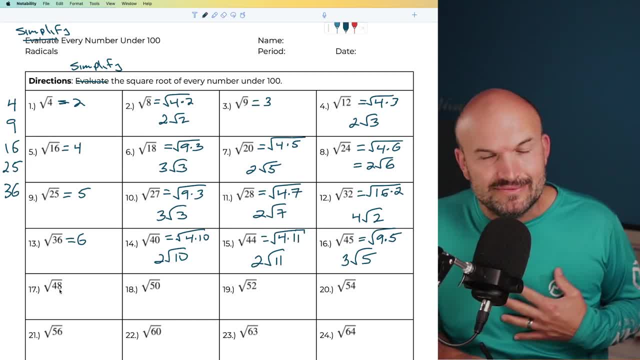 48. Again, initially I think of four right, Cause it ends in an eight. but then I was thinking, is there a larger number Right? And again, sometimes you can work your way backwards, like 36. Now that doesn't go 25. No 16. Ah, 16 does work, Right. So again, sometimes you might. 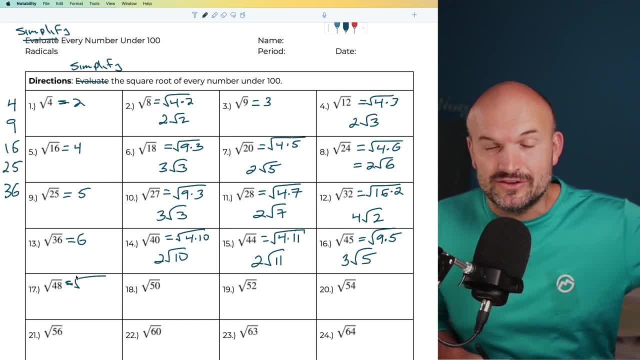 have that initial thing like: Oh, four is usually going to go into it, but is there a number higher than four, a square number that evenly divides it? to that, In this case we do have. we have a 16 times a three square to 16 is going to be a four. 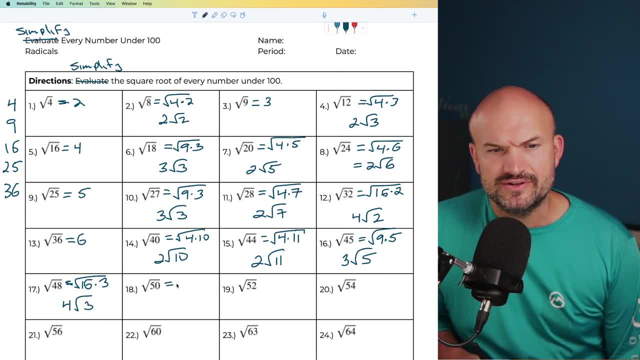 Times square root of three here at 25.. Um, I know it was going to 50 or I can rewrite that as a 25,. um times two square to 25 is going to be a five square root of two. And then for this one here now, this one you can start kind of taking with like number 19.. 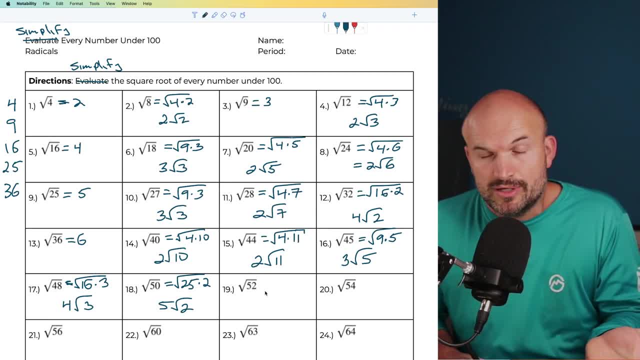 What you can do is like start thinking of this as like, dividing it by two, right, That's an even number. So if you divide it by two, right, that's going to be a 26. divided by two again, Um, that's going to be a 13.. Oh, 13 times four, right, Cause you divided it by two. 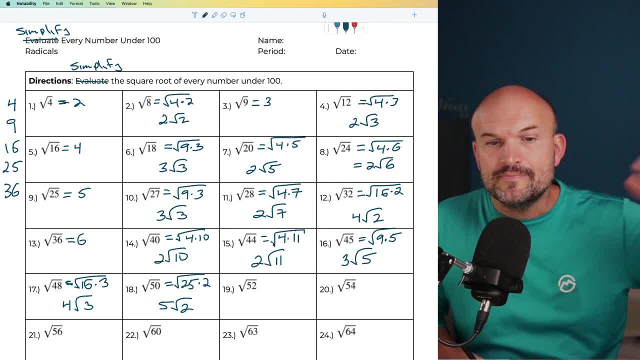 which is technically divided it by two twice, which is kind of like dividing it by four. So even if you don't know initially, like how many times is four going to 52, just keep on dividing it by two, That's, and then you'll see like Oh, two went, divided by two twice was same. 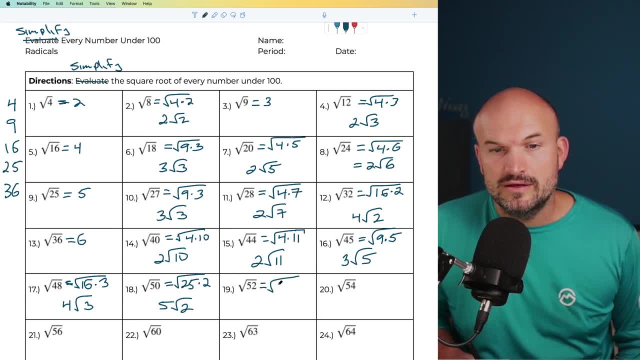 thing as divide by four, So therefore I can rewrite this as a four times a 13, and square to four is going to be a two times a square root of 13.. Uh, next one over here, this one's even, but again. 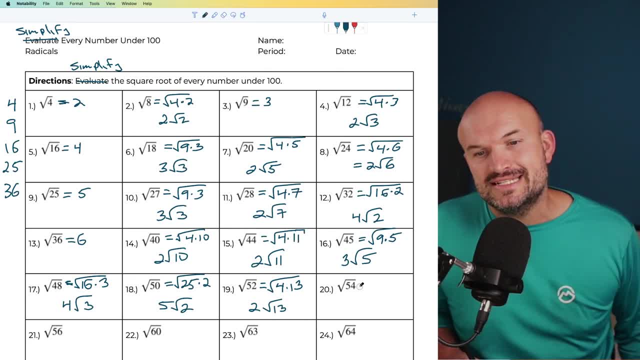 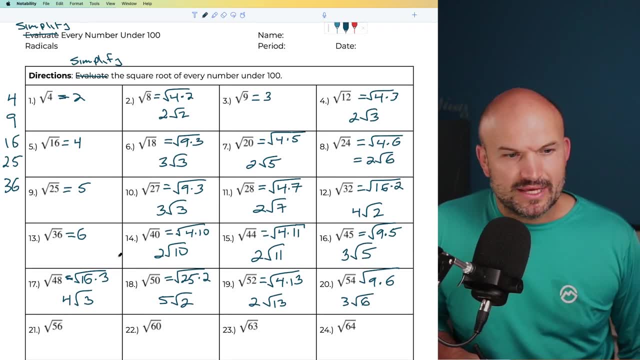 hopefully, you recognize, you know your multiples of nine. you recognize. Oh, this would be nine times a six. So I have a nine times six, Um, so therefore, that's going to be a three square root of six. Okay, Um, again the same thing I'm going to do over here. I'm going to divide this Um. 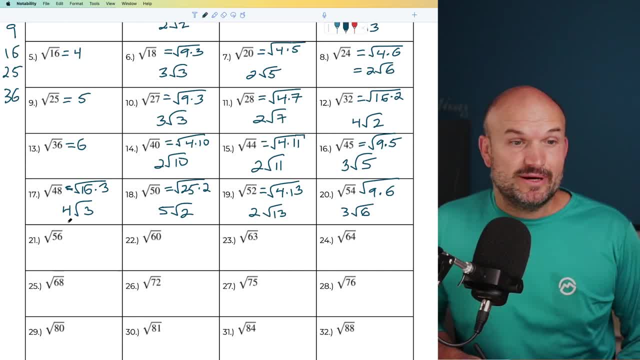 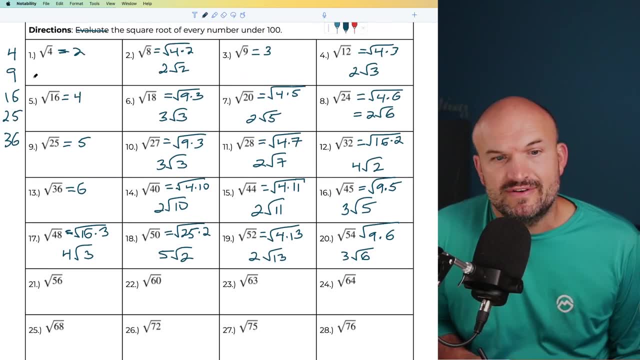 like see: if you divide this by two, that is going to be a 28. divided by two, Again, that's going to be a 14, right, Um, and 14 cannot be simplified any further. There's no other square numbers that you can divide into um a 14.. So, therefore, that is going to be the 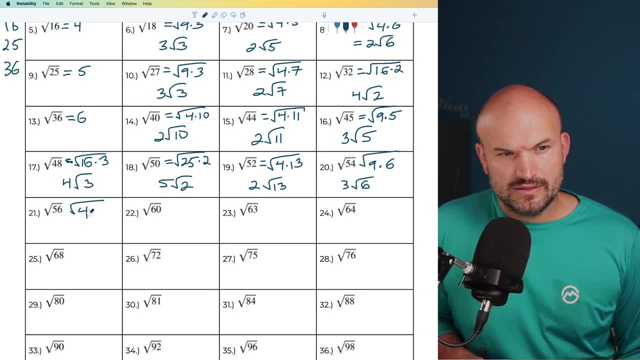 next one. So let's see, I can rewrite that as a four times a 14.. Over to four is going to be a two square root of a 14.. Um, again 15,. hopefully you recognize 15,, 60,, um, or, or, I'm sorry, going again through this, I recognize that 15 divided by 30 divided. 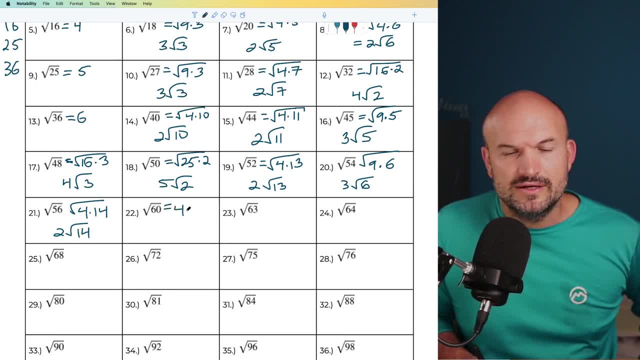 by two, Again it's going to be 15.. So therefore I can rewrite this as a four times a 15, and square to four is going to be two times the square root of 15.. Now here I recognize an odd and I say: 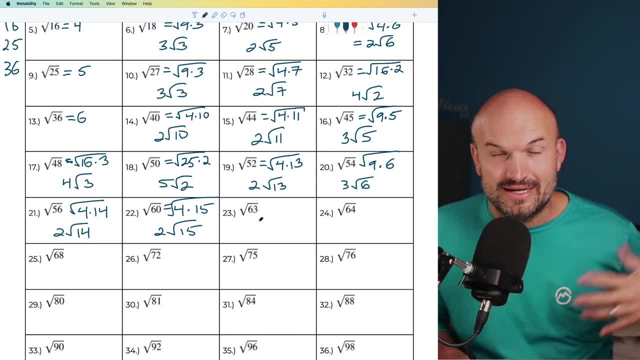 Oh yeah, Nine. does nine go into 63.. Oh yeah, Seven times. right, Or yeah, seven times. So therefore, I can rewrite this as a nine times a seven square root of nine is going to be a three square root of seven. Um, did I miss a couple? I think I did 36.. Where did I get to? Oh, my God, I did forget. 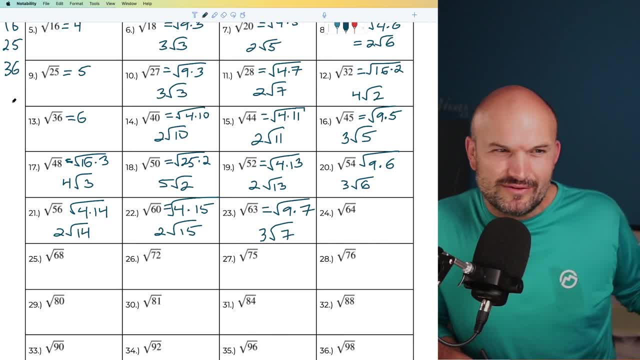 49.. Holy crap, Let's go ahead and do it. I was wondering about that. I'm like: where'd 49 go? So I'd forgot to type that in Shoot. Okay, Well, let's go and add 49.. Then there's a 49 that goes. 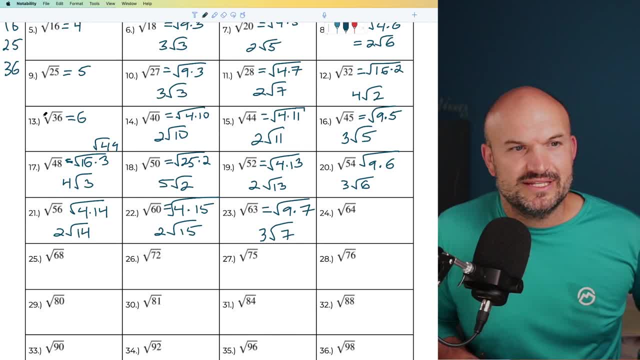 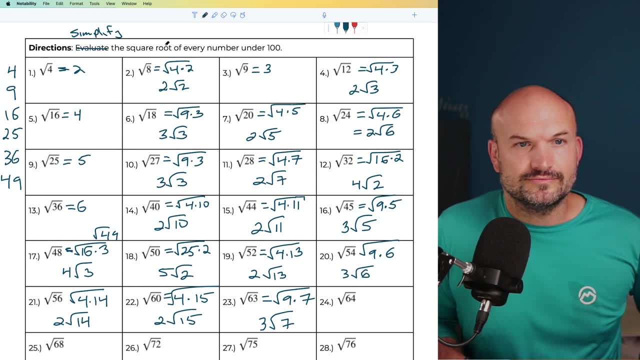 into there, guys. So square root of 49, I must've missed that square number. So we have 36 and we have 49, which is another square number, right? Because, um, let me go ahead and write that up there. Um, square root of 49 is going to equal seven. So I will update the sheet for those of. 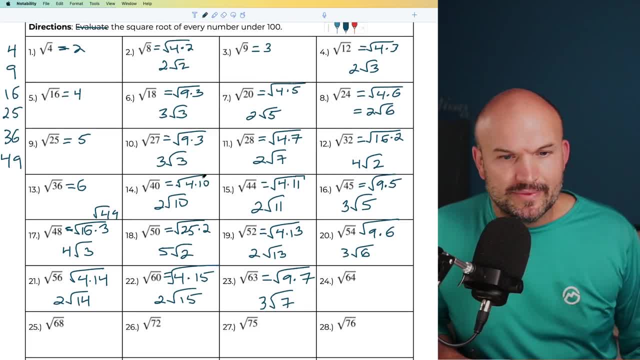 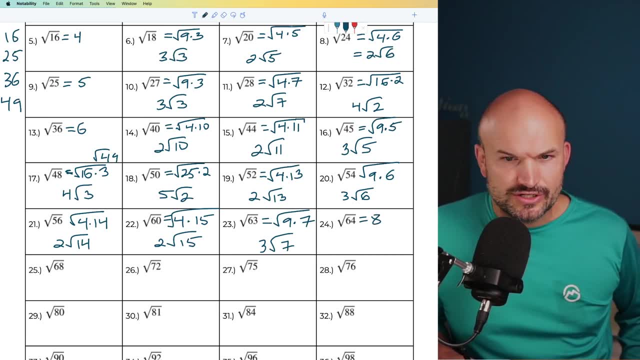 you that are following along from that. I can't believe I forgot about that Um. all right, So then we have square root of 64, which is going to be an eight Um, and then let's go and get into. 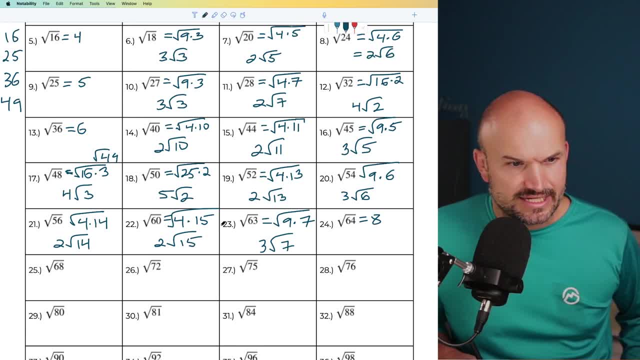 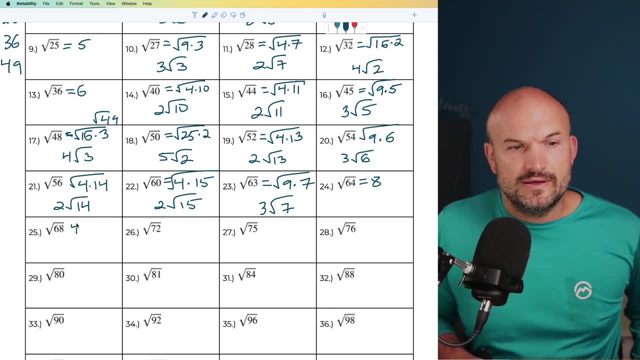 okay, so now we have 25, which is going to be a 68.. Okay, So, again, we divide by two. um, it's 34, divided by two, Again, it's going to be a seven. So you could say: all right, so let's say four times a 17 square to four is going to be two. 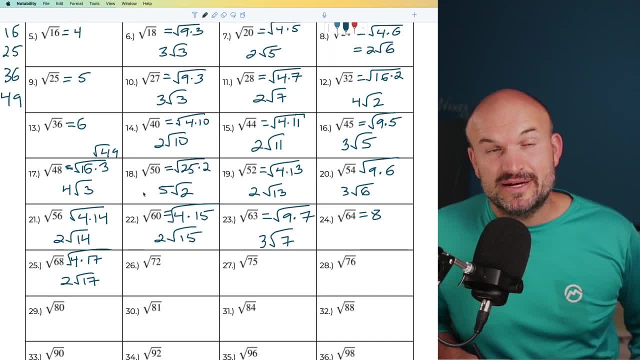 times a square to 17. here I recognize um again, divided by two is a 36, right, Oh, 36 is a square number, So I can rewrite this here as a 36 times two. A lot of people might say, oh, can't you do. 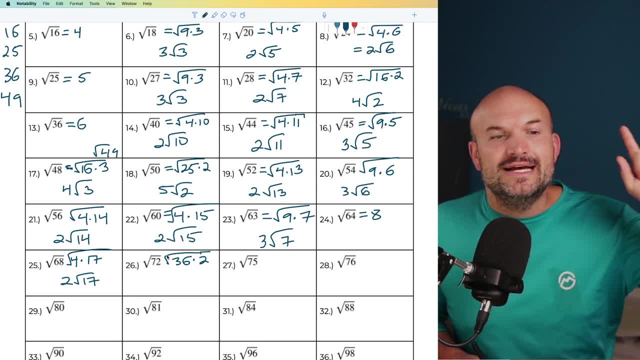 nine times eight. Yes, of course you can Right, But again, guys, our goal is to do the largest number, largest square number that evenly divides into that term Um. so therefore we have a a um 36.. Well, that's going to be a six times a square root of two. here I recognize a ends in a. 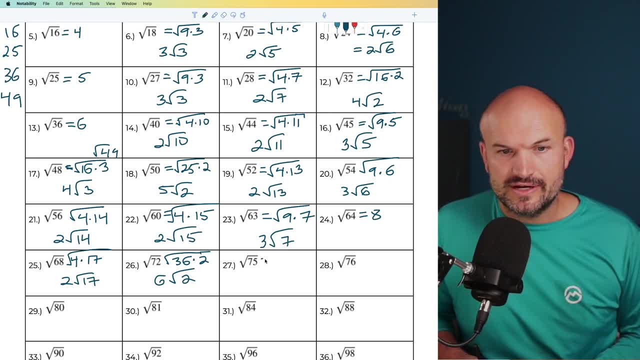 five, 75,, 25 goes into there three times, So I can rewrite this as a 25 times three, square to 25.. It's going to be a five times a square root of um three, And then this one I'm going to divide. 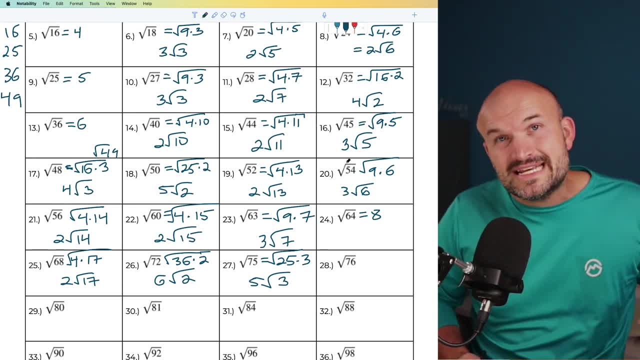 out. Um, I'm not sure what 76 starts to get big numbers right, But I know it's even so. I can divide it by two. um, divided by two, That's going to give me a 38, uh, divide that by two Again. 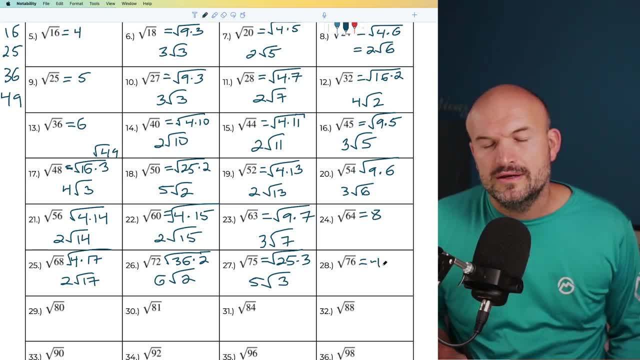 that's going to be a 19.. I'd say, oh, okay, So I can rewrite this as a four times. Let me fix that up So this could be a four times a 19.. There you go, And the square root of four is going to be two. 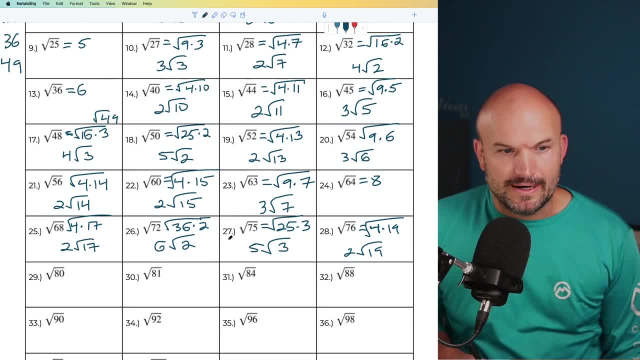 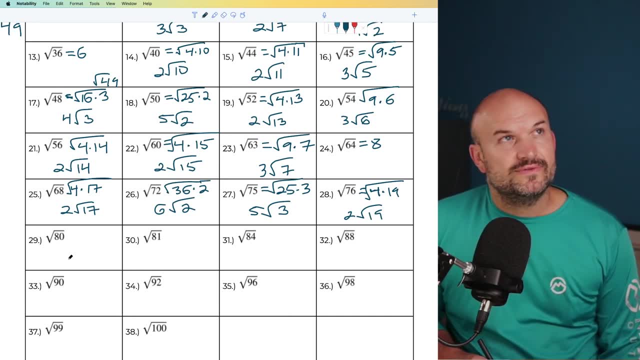 times a square root of 19.. All right, now let's go and get into our 80,, which is going to be: um, let's see here. So, thinking of 80,, um, I recognize that. let's see here. And now I know. 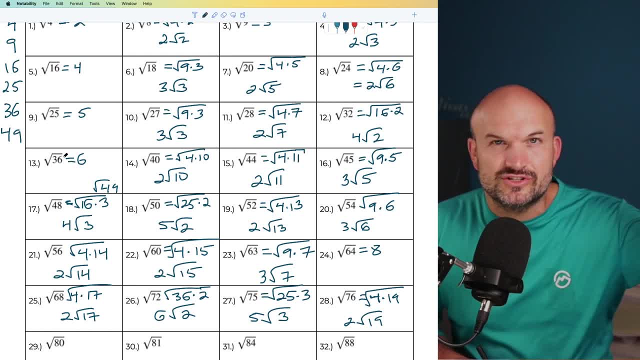 four is going to go in there. I'm going to go in there. I'm going to go in there. I'm going to go into there 20 times, right, But then I can reduce the square root of 20, right, If I think. 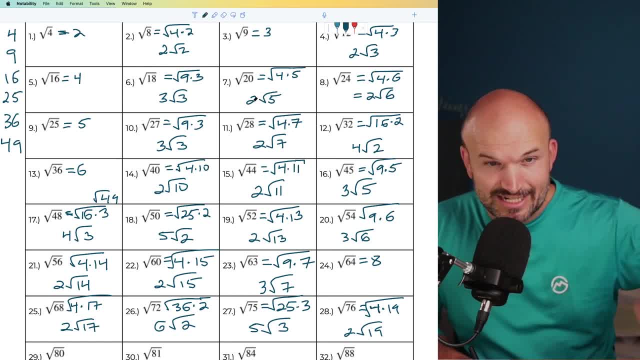 about a square root of 20, that's going to be um a two times five, So that'd be already. you're going to be multiplying that Um, so then the two times four, which is going to give you or two. 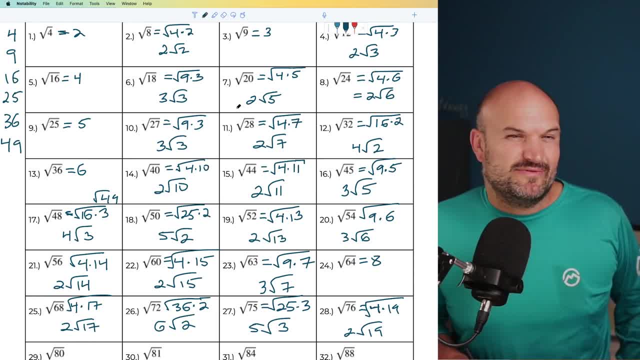 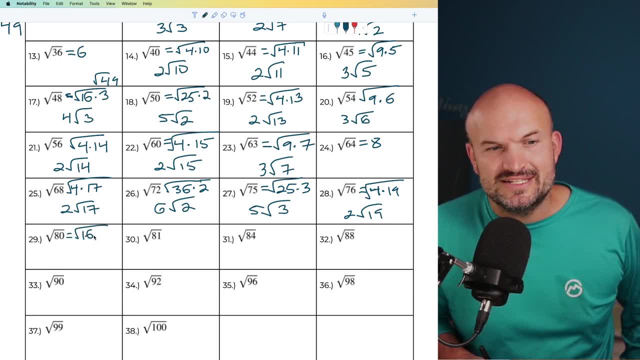 times um two, which would give you four. So I'm actually giving: your final answer is four times square root of five. but let's see that means what this is. So I'm kind of doing my mental math in my head. This can be rewritten as six. How many times is five going to there? Well that's. 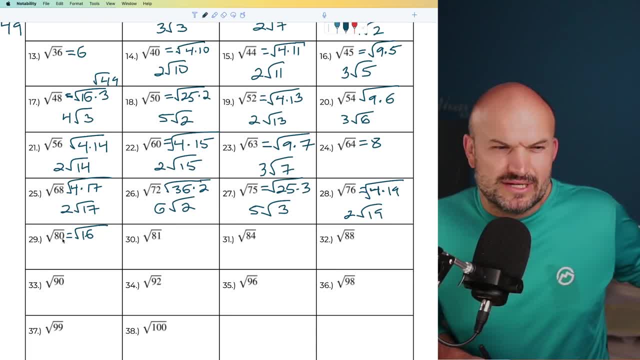 going to be five, goes into 50, 10 times, And then it's going to go in there four times. Um, yeah, 10 times, And then, I'm sorry, there's an extra 30. So it'd be six. There you go. So 16 times five. doing some mental math in my head. 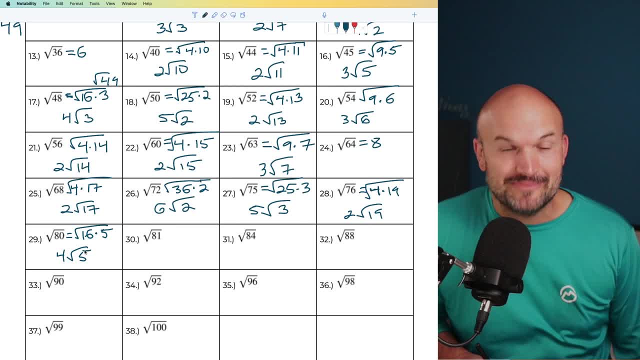 Don't bother me. Square root of 16 is going to be a four, square root to five. I'm sure none of you have tried like doing all of these problems all at once, Like it's such a great idea. Um oh man. 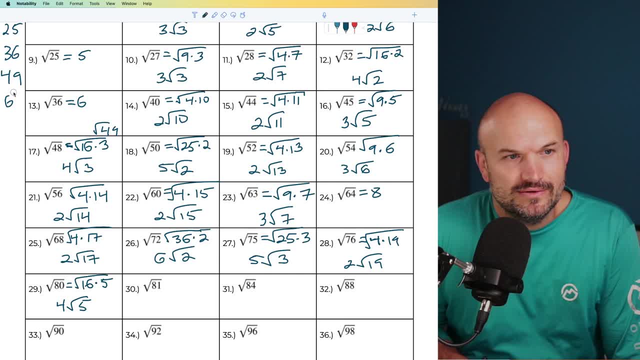 Okay, Ooh, And the next square number. why do I keep on forgetting? So we have 64.. That was a square root of eight. I forgot to write that in there. Sorry about that. Then the next one: we have nine, right? So square root of 81 is going to be a. 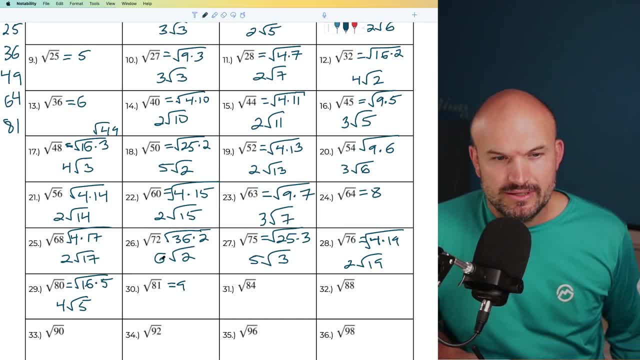 nine, So that's going to be 81,, which is our next square number. Um, then we have our 84.. So, okay, So let's divide that by two. Um, that's going to be a 42 divided by two Again. 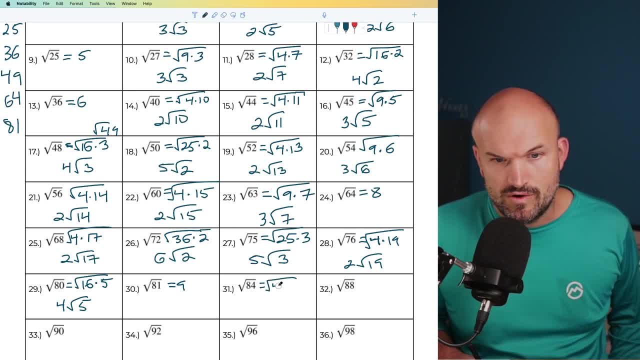 that's going to be a 21.. So, therefore, I can get that. as to a four times a 21, square to four is going to be a two times a square root of 21.. Then we have a 32.. Um, again, we can do the same thing. 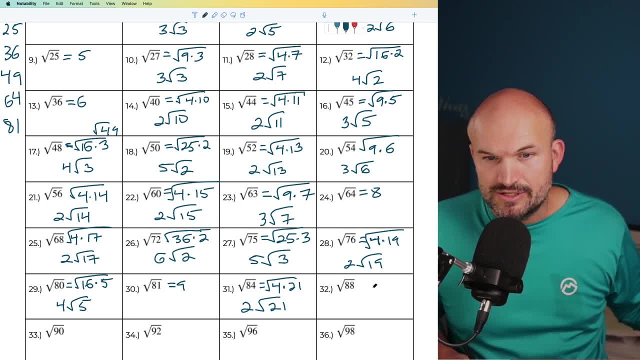 divided by two, is going to be a 44. divided by two, Again, it's going to be a 22,. right? So therefore I can do a four Times a 22.. So notice, if I don't know exactly, there's already a bigger number that knows. 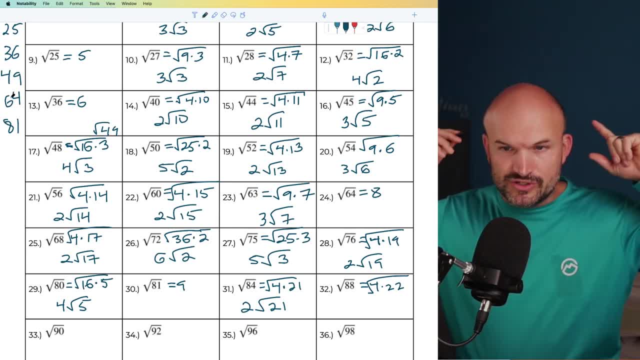 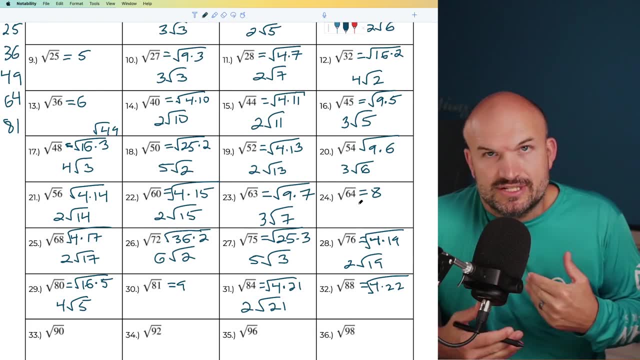 evenly into it. I kind of work with my prime factorization to divide it by two, um, to kind of see what is going to work. And a lot of times, if anything else doesn't work from that case, then I'll just, you know, divide by two in that case, to see what I can do. 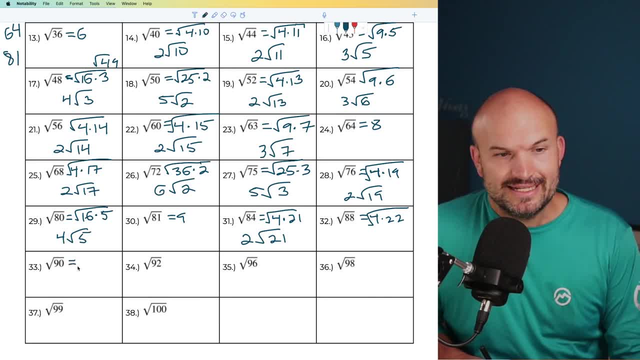 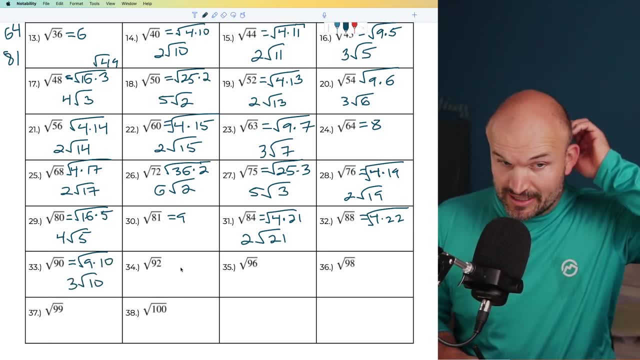 Um, all right. So nine times 10, well, I know, nine obviously 90.. So that one's going to be a nine times 10 square to nine is going to be a three square root of 10.. Um, now, this one could. 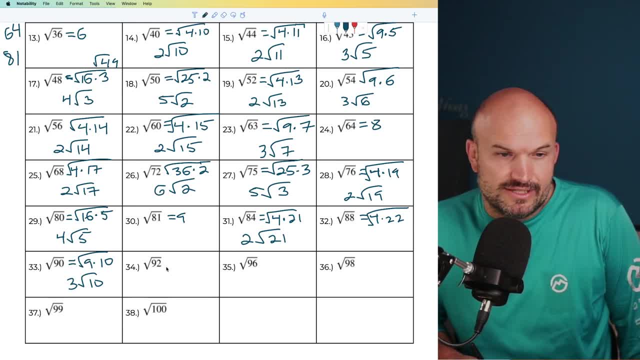 be a little bit of interesting. So, um, it's even right. So let's see, that would be a 46. And then if I divide a 46 again, that'd be a 23. So again, I'm just divided by two twice, which is technically divided by four. 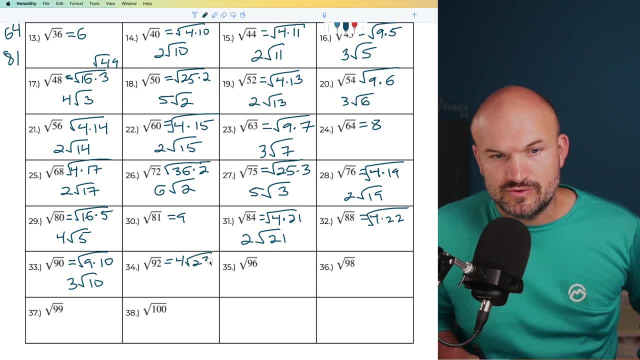 So therefore I can say that's the same thing as a four times a square root of 23.. Um, oops, I'm sorry, Let me fix that correctly. You're rewriting it under the radical as a four times a 23.. And then square root of four is going to be two times the square root of 23.. 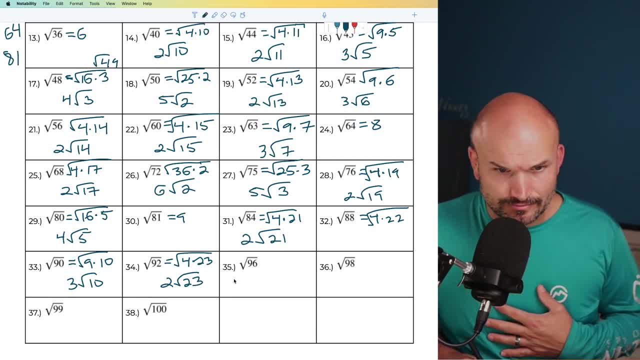 All right, Now we have our 96, um, which again I'm thinking into this one. Like I don't think I need to divide by four, 96 sounds like a pretty common number. And again, if I'm thinking about 96, um, that was already half right of 48. And I know 48 can be divisible. 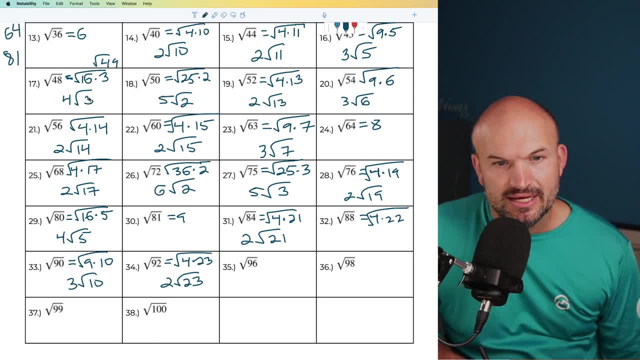 here. So what I'm looking into is saying: all right, well, that's going to be. what else can I simplify there So that one 16 went into there three times. So if it's not double, that means this could be written as 16 times a three times right. So therefore I can re. I'm sorry. 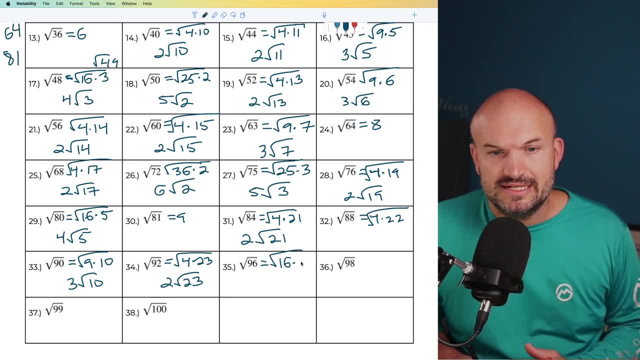 16 times six. So therefore I can write this as a 16 times six. square root of 16 is going to be a four square root of six, um 98.. Hmm, Uh, let's go and see if we can do a square number here to: 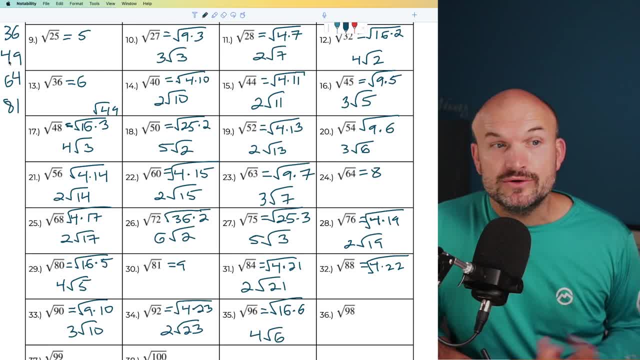 what if I doubled 49 died too right, That's getting to be 98.. So that one's kind of actually easy. So therefore I can rewrite this as a 49.. Come on, write your 49s correctly. So this would be a 49 times two square root of 49 is going to be a seven square root of two. 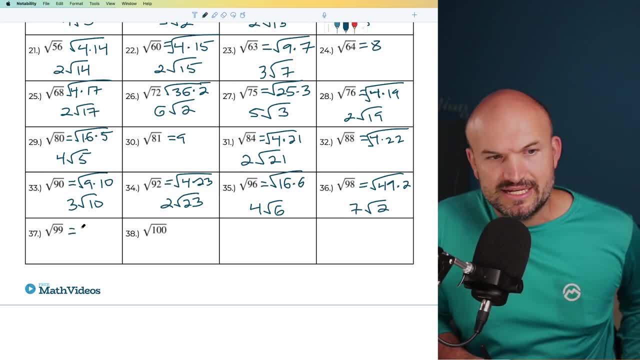 Um and 99, that's going to be a nine times 11.. That one's kind of easy. So this one would be a square root of nine times 11. square root of nine. It's going to be a three times square root 11.. 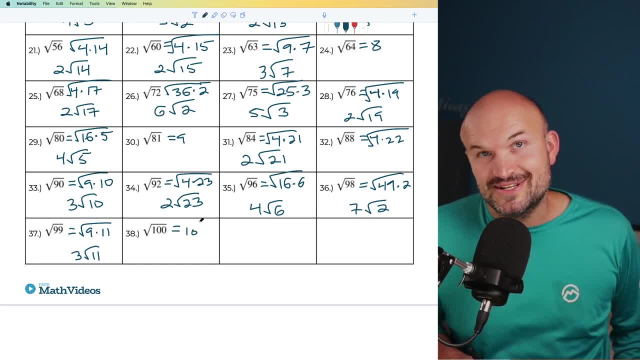 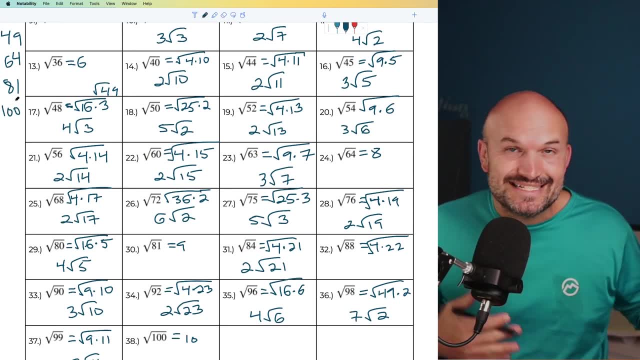 And then we have, last but not least, guys, is the last square number under a hundred, or at least over a hundred, with equal to a hundred, which is going to be a 10.. So therefore, ladies and gentlemen, that is all of the numbers, that you can go ahead and simplify the square root, A lot of these. 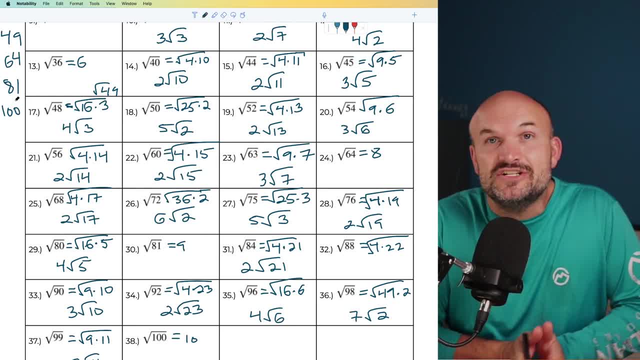 I did not work through very um very slowly. So if you want any individualized examples or maybe even some higher numbers, then check out the next video I have for you here. Cheers.